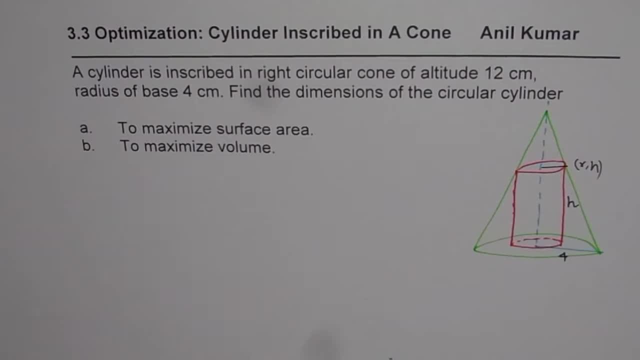 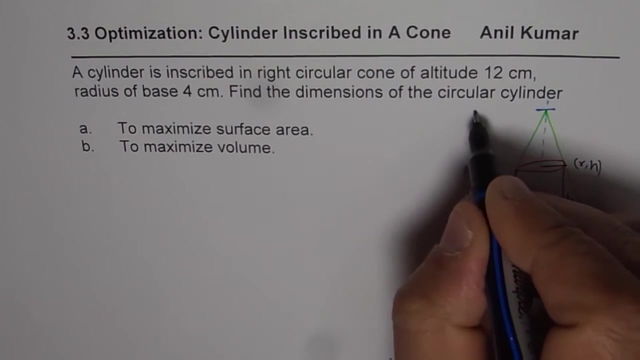 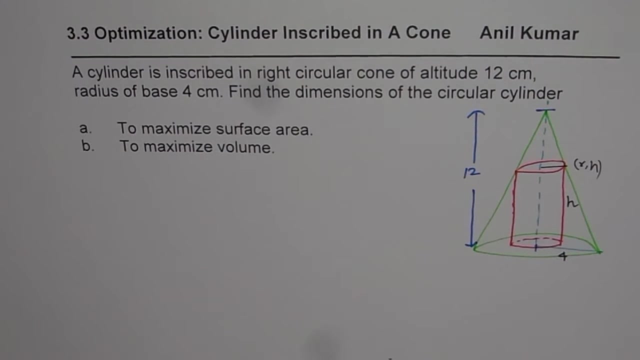 cylinder is h, So those are the dimensions which we need to figure out as far as the cylinder is concerned and for the given cone. we know that this height is 12, so this is 12 for us. let me write 12 here, so that is 12, and 4 is the base right, so that is 4. so these dimensions are given to us for the cone. 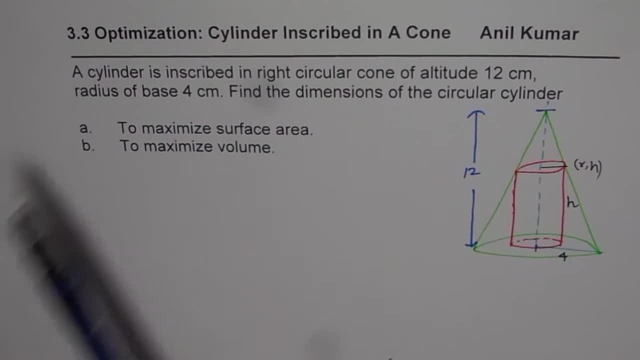 we need to maximize surface area. that is part one, and then we'll also see how to maximize volume. the reason of taking both of them together is that we have almost the same strategy. right strategy here is we are working with two variables: radius and height. we need to find relation of one. 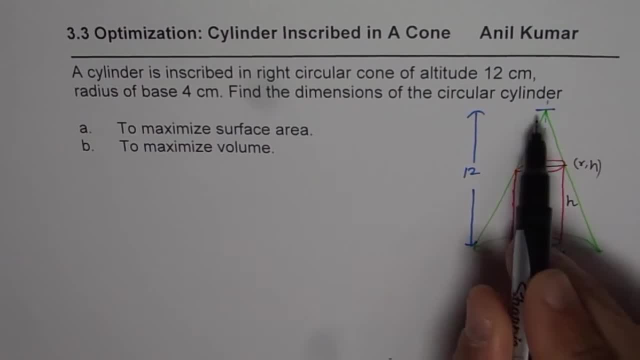 variable with respect to the other. how do we do that in this scenario, whenever a cone and a cylinder are involved? now, the best way to do it is look into triangles which are similar you. so let me say this: let me label some pranks this: a, b and c, so that big triangle is similar to. let me. 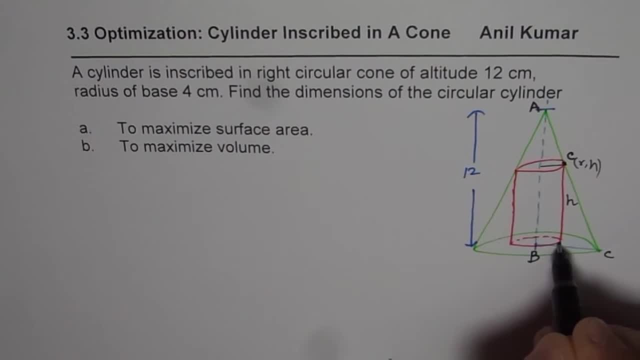 call this point as c and this point here as d, right? so if you consider the triangle big triangle a, b, c, you'll find that this triangle is similar to a triangle. i mean, let me call this e, right? so c, d, e, these two are similar triangles. why so? now, both of them the big triangle. they're right angles, correct. 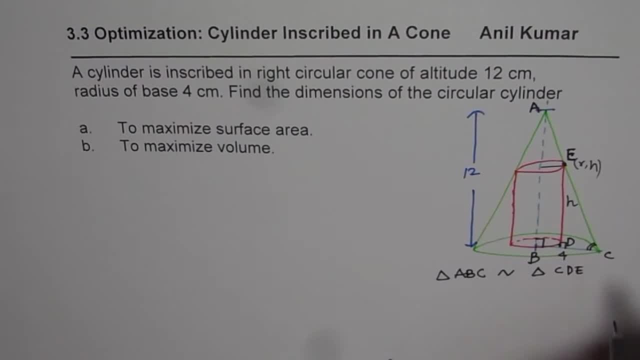 so this is right angle. plus, we have this common angle. do you see that? so a, a property, so we say property which is double, a right, so that is the property which makes them similar. now, when these triangles are similar, in that case ratio of sides will be constant. so that means that we have a. 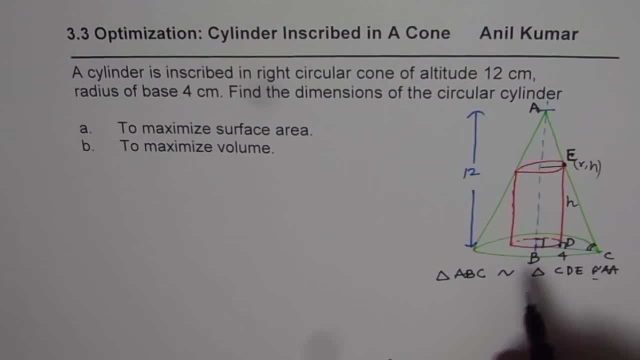 constant. so ratio of sides will be a- b. big triangle: a- b is 12 divided by b- c, which is 4 for us, should be equal to e d, which is h over d c. now d c is 4 minus r, since this is r for us, so this is r, so 4. 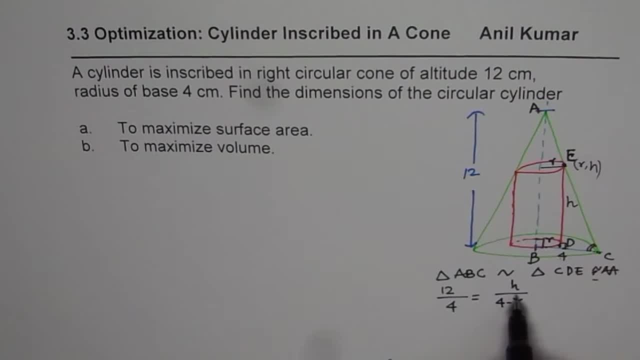 minus r, 4 minus. so that gives you a relation between h and r. so this is 12 divided by 4 is 3.. We can write this: So h is equal to 3 times 4 minus r, So that becomes the relation between. 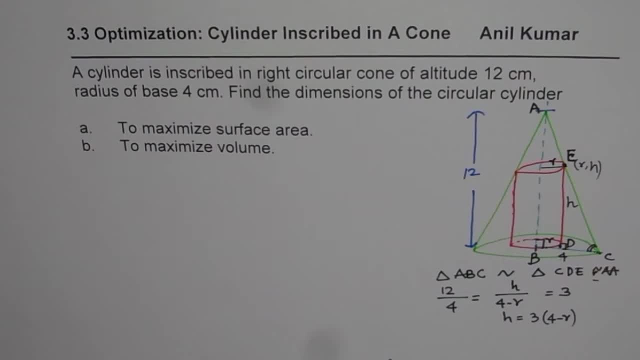 h and radius. So first part is find the relation between the two variables you are working with. So once we have found this, we'll say: let this be equation number 1.. And now we will see how to maximize surface area. Now, what is the surface area of the cylinder? So let's start with part a. 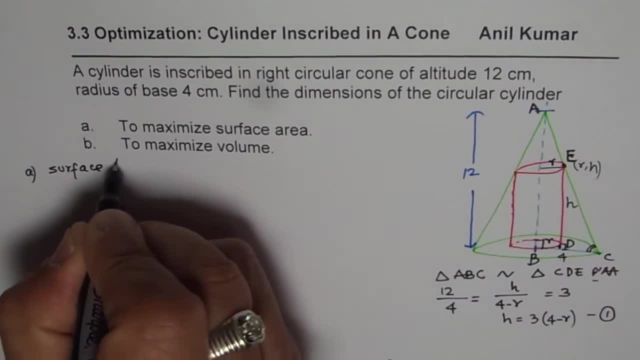 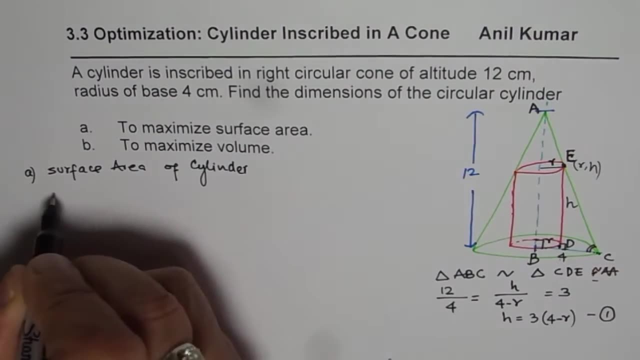 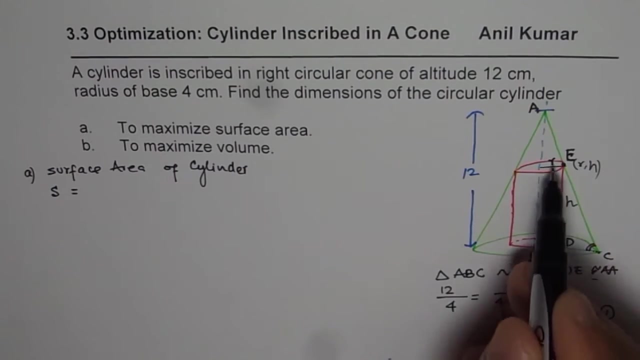 which is surface area of cylinder. Now, surface area of cylinder, let's say s, is equal to: there are two surfaces on the top which are circular, top and bottom. So it is 2 times pi r square plus lateral surface, which is 2 pi r times h, 2 pi r times h, right. 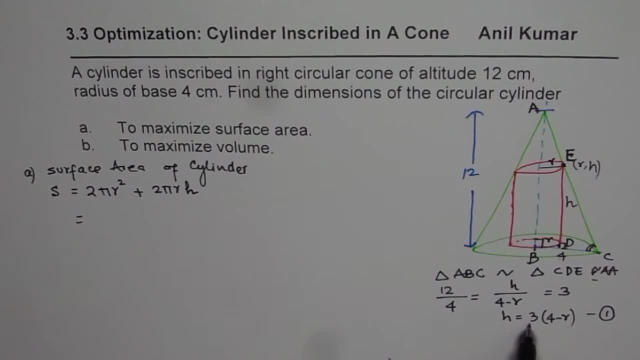 Now, surface area of cylinder is 2 pi r times h. So let's say 2 pi r times h. So let's say 2 pi r. since we already have a relation for h, which is 3 times 4 minus r, We can substitute h with: 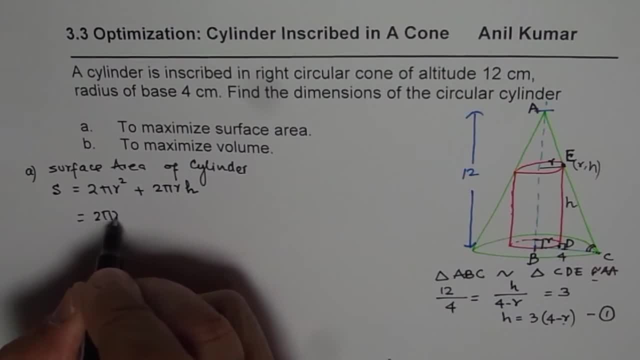 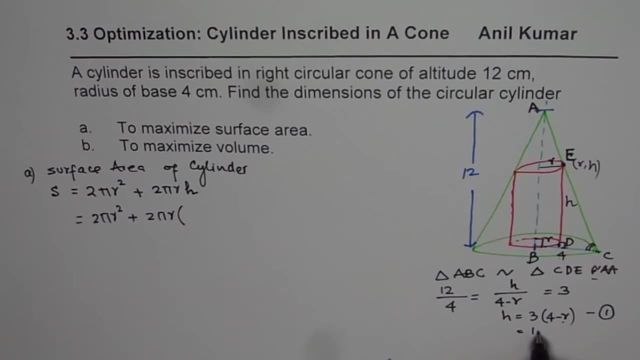 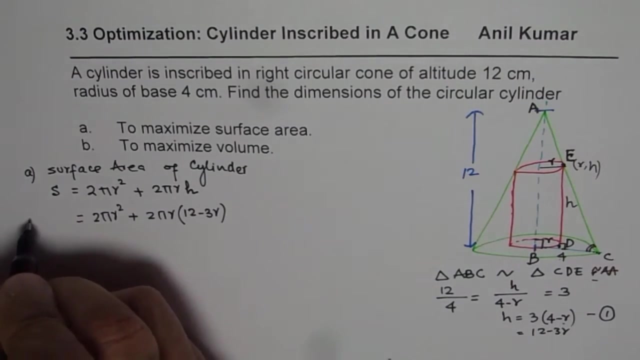 this value, So we get 2 pi r square plus 2 pi r times. Let me write this as 12.. Let me write this as 12 minus 3 r, So we get this as 12 minus 3 r. So we got surface area in terms of r, So single. 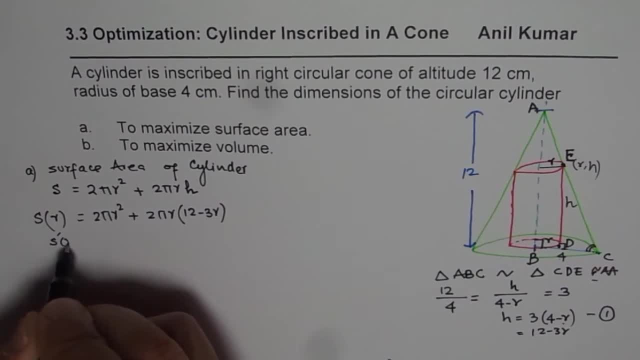 variable. Now we can substitute h with this value, So we get surface area in terms of r. So single variable: Now we can substitute h with this value, So we get surface area in terms of r, So we can find the derivative right to maximize. So that will give us a critical point. So which will be? 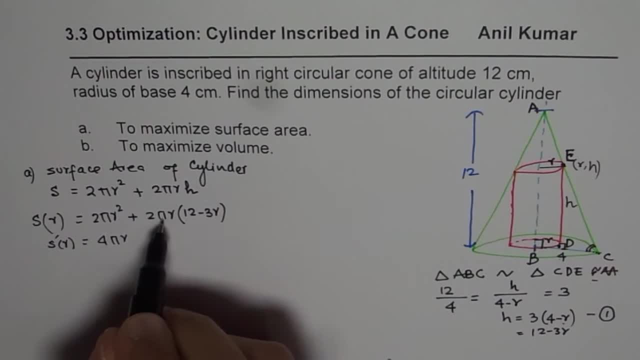 4 pi r, and when you multiply this we could say 2 pi r, 2 pi times. let me do product now: 12 minus 3 r, plus derivative of inside function times: 2 pi r, Inside function is minus 3, right. So so it's a. 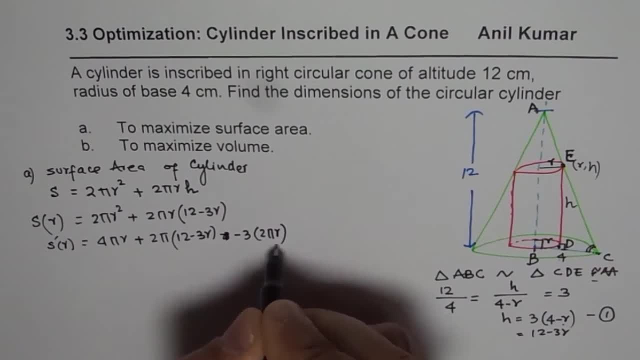 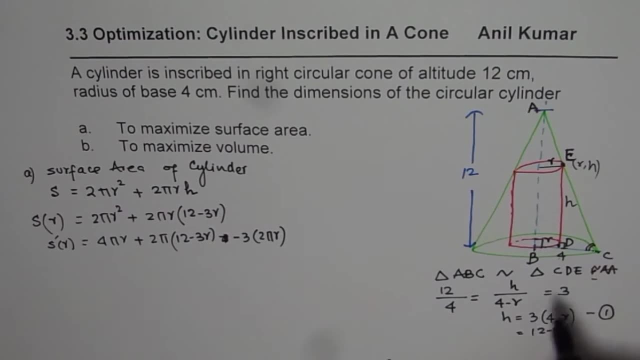 minus 3 times 2 pi r, So that becomes the derivative. We used the product rule here, correct? Now what is the limit for r? in this particular case, As you can see, r could be from 0 to 4.. So r is either greater than equal to 0 or is less than equals to 4.. So these are other. 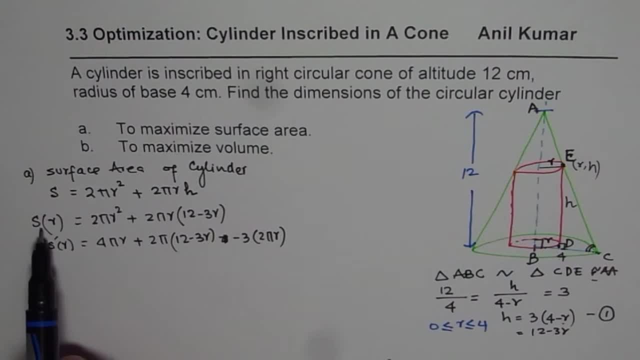 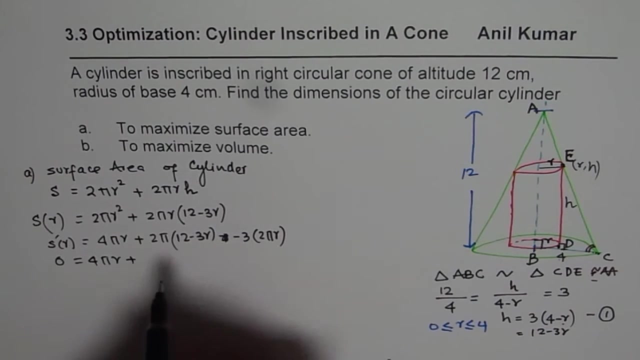 boundary conditions which we could test surface area at. So if I write 0 here, then I'll get that expression, which will be 0.. So we know s Let's find the critical number first, and then, if I equate this to 0 and solve for r, what do I get? So let me expand this: We have 4 pi r plus if I 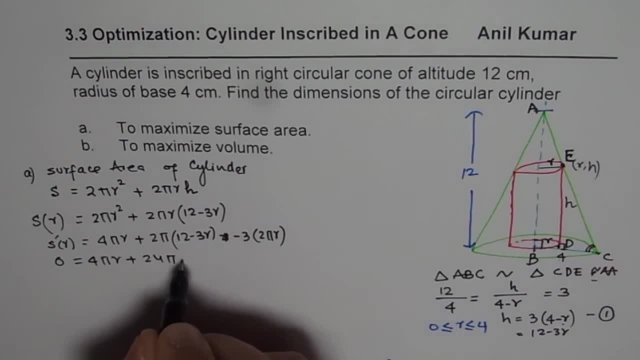 multiply by 2, 24 pi minus 3 times 6 pi r and here 6 pi r, correct. So that becomes the expression Now combining the terms 4 pi r minus 6 pi r is minus 2 pi r, So we: 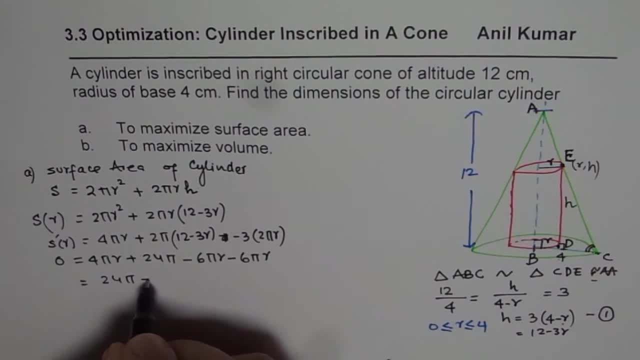 get minus 8 pi r. So 24 pi minus 8 pi r equals to 0, and from here we get r as equal to when you equate this, So we get. or you can write one more step: 8 pi r equals to 24 pi or r equals to 24. 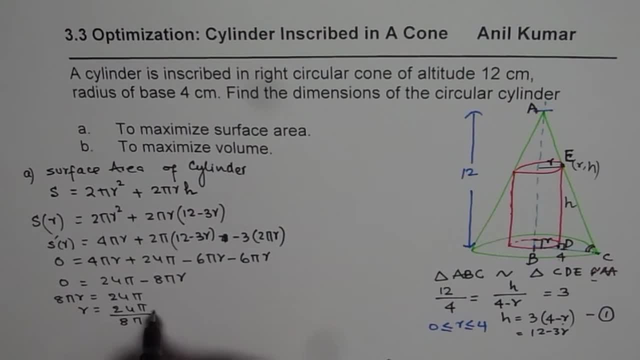 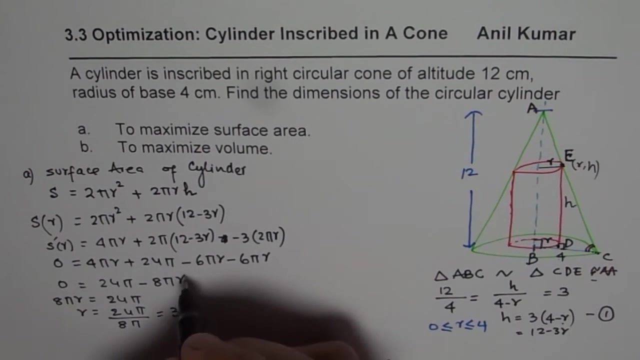 pi divided by 8 pi. So 8 goes 3 times, So r is 3 for you. So in this particular condition, we get r equals to 3 for a maximum surface area of a cylinder. Now, as an exercise, what you can do is: 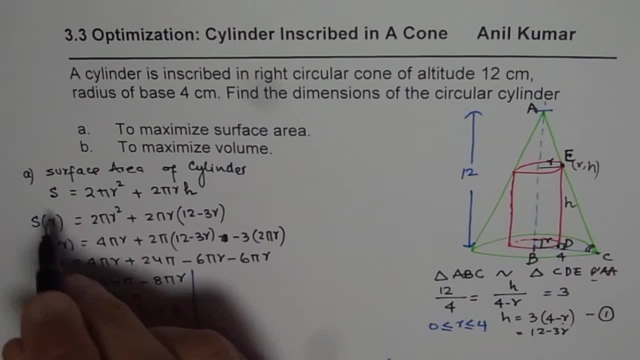 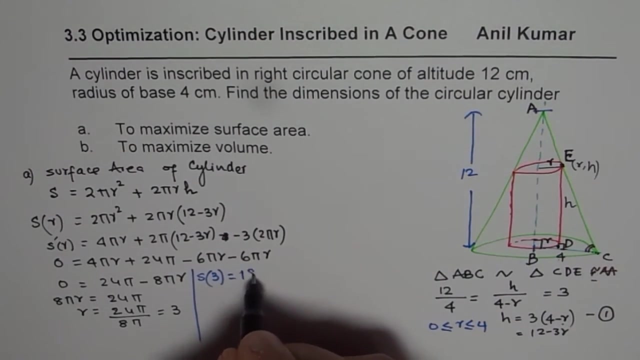 you know surface area, Find surface area s for 3, right? So calculate this value. So when you plug in 3, you will get your answer right. So it is 2 pi times 3 square, which is 9 times 2 is 18.. So I am just writing 18 pi here plus. we will use this. 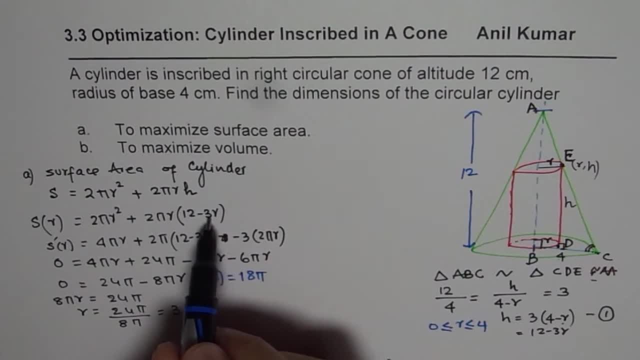 expression, since I know r here: 3 times 3 is 9 and 9 minus 12 is 3.. 3 is 6.. 6 times 3 is 18.. So 18 pi, right? So plus 18 pi. 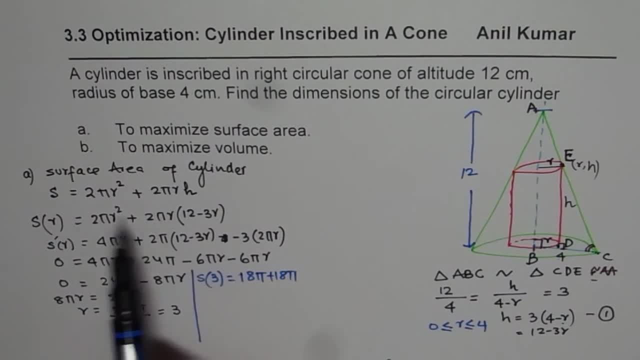 So just substitute here value of 3.. Calculate s of 3. So 3 square is 9.. 9 times 2 is 18.. So we get 18 pi from the first term In this case. if I put 3 here, 9. 12 minus 9. 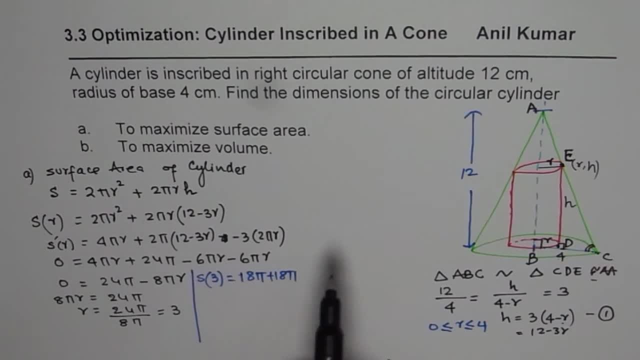 is 3.. Here it is 3.. 3 times 3 is 9.. 9 times 2 is 18.. So we get s of 3 as 36 pi. So that becomes the surface area in centimeters square. Perfect, If you substitute s of. 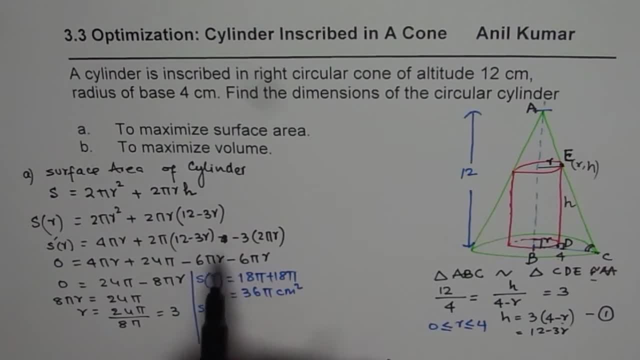 0, you'll find that to be 0, and if I substitute ss4, that will also be- and that is equal to s of 4, which is equal to 0. so from here you can say: maximum is at r equals to 3. to maximize surface: 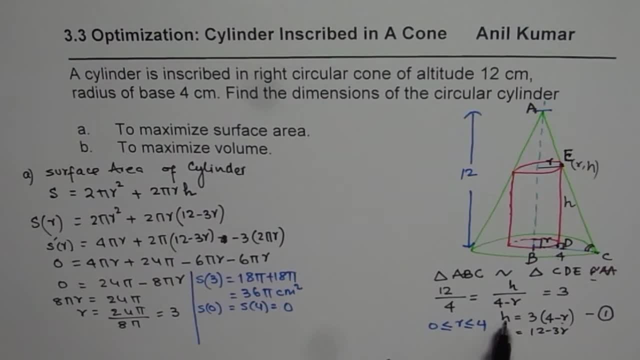 area. the dimension should be r is 3 and you can find what h is. so h will be equals to, if I write 3 here, 4 minus 3, so I get 3 times 4 minus 3, which is indeed 3 itself, right? so for the first. 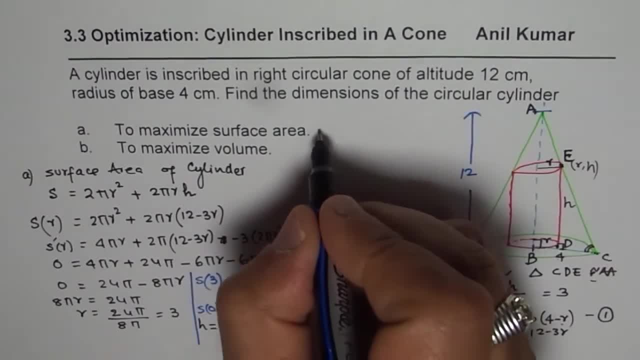 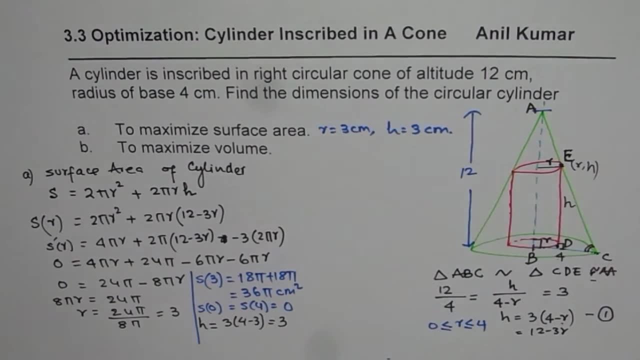 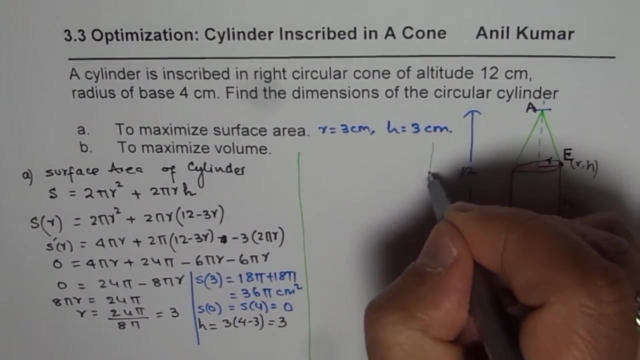 part we get our answer to maximize, we get r equals to 3 centimeters and h equals to 3 centimeters. is that okay? so that is how you would solve this particular question, right? so we have done part a. now let us look into part b, right? so I'll do part of it now. you know the 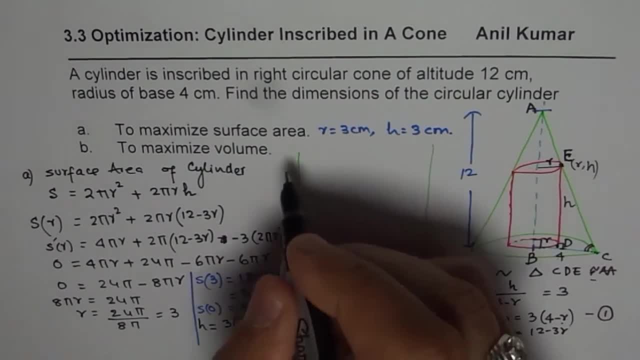 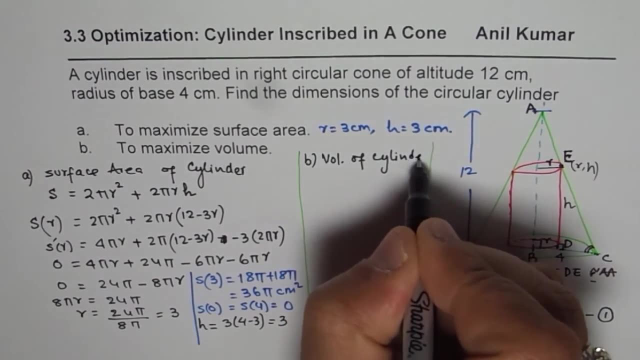 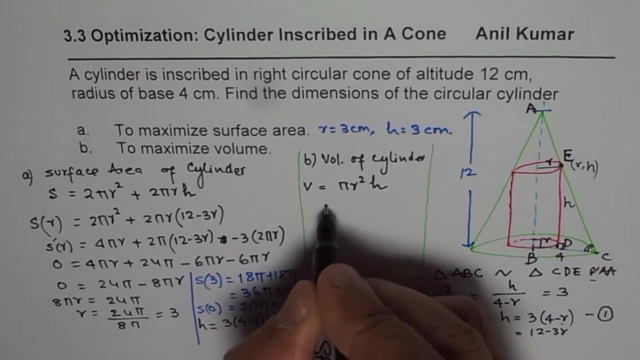 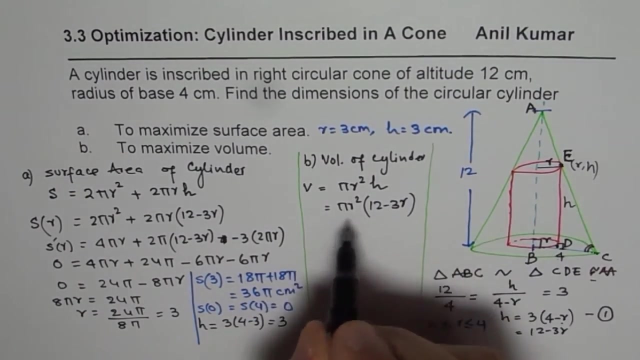 how to solve it. So what is the volume of cylinder? So now we are considering part b, which is volume of cylinder. So volume is pi r square h. h we already found as equals to pi r square h could be written as 12 minus 3 r, 12 minus 3 r. This time I will actually expand. 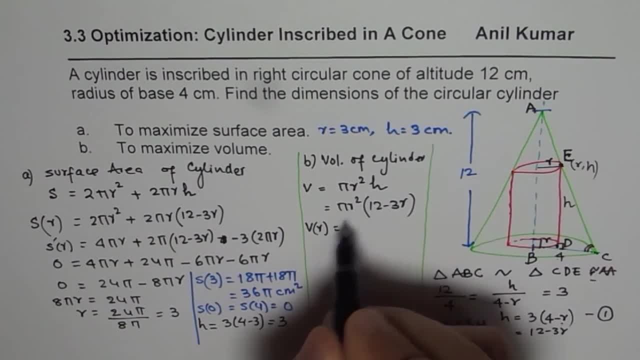 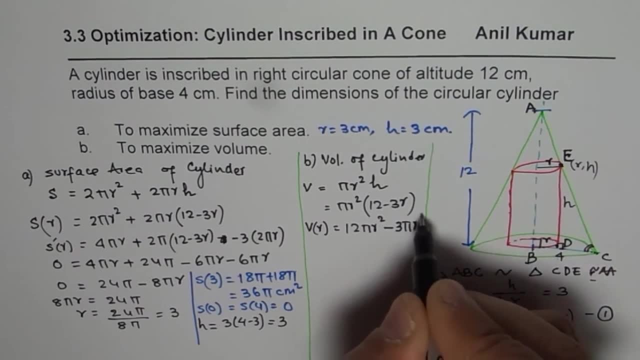 this It becomes kind of simpler. So if I expand we get 12 pi r square minus 3 pi r q. Derivative of this function volume is 24 pi r minus 3 times 3 is 9 pi r square, So that 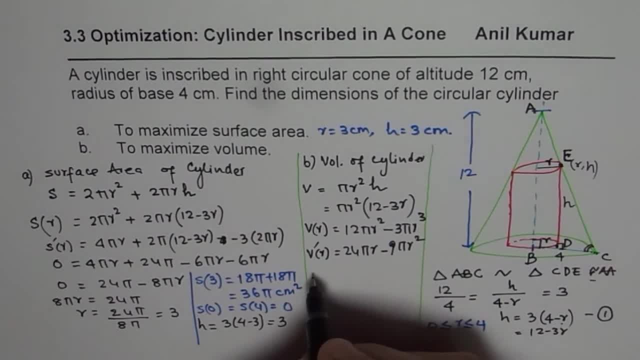 becomes the derivative. Now critical point will be when this is 0. So that means 24 pi r minus 9 pi r square, and to equate them to 0 we will get r is equals to well. let me just take it on the other. 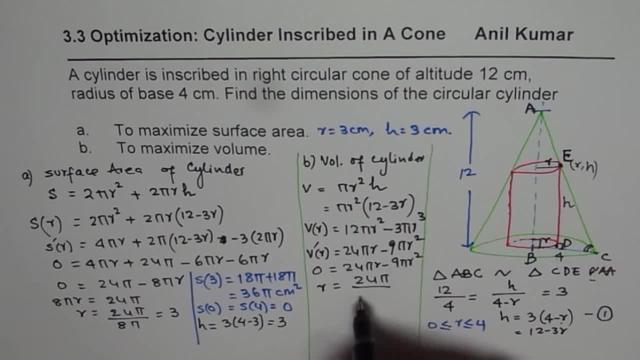 side 25 pi divided by 9, pi right. So pi and pi cancels. and you can simplify this dividing both by 3.. So we get 8 over 3.. So radius will be 8 over 3. for maximum volume You can substitute 8 over 3 in this expression: 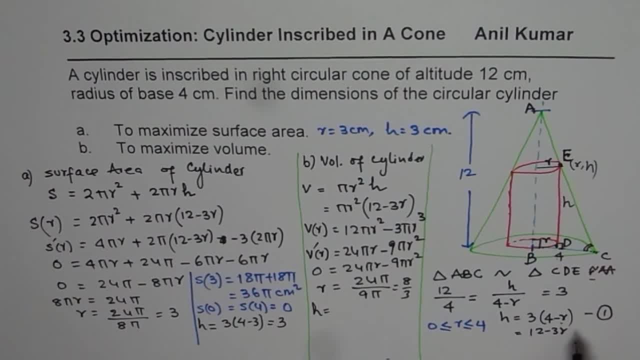 to find height. So height will be equals to 12 minus 3 times 8 over 3, which is 8.. So that means 4.. So for maximum volume, the solution is: r equals to 8 over 3 centimeters and height. 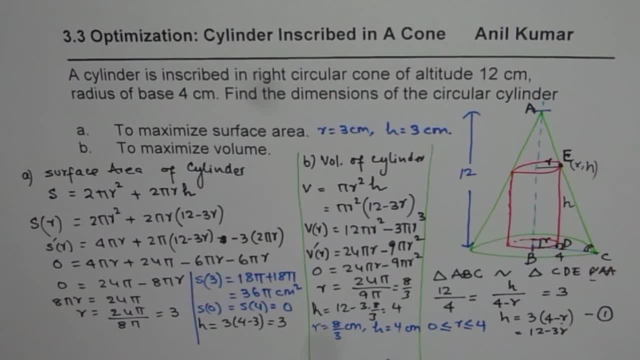 is 4 centimeters. So in a short space and in a shortcut kind of method, but complete details- I have shown you how, when a cylinder is inscribed in a given cone, we can solve for maximum area and maximum volume, right? So obviously the size are very different, right? But what you will,